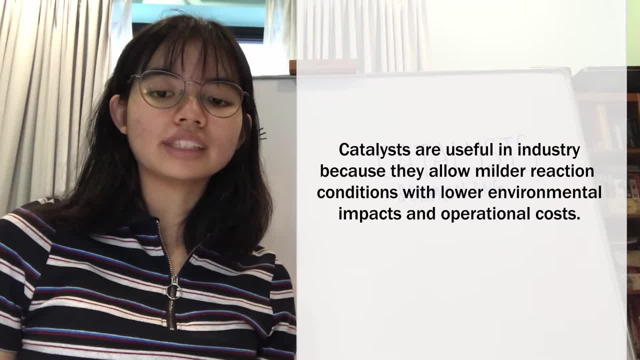 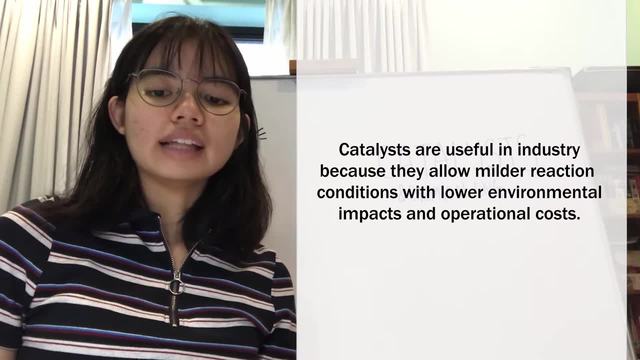 be carried out under milder conditions, with less energy needing to be supplied to the reaction. For example, the reaction might be able to be carried out with a lower temperature, which saves electricity, and this saves operational costs as well as reduces the environmental impact. There are two main 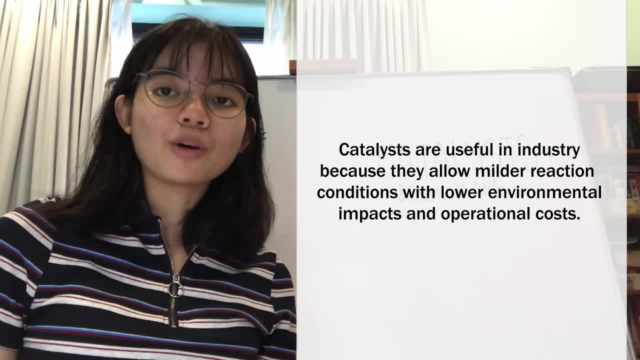 types of catalysis: heterogeneous catalysis and homogeneous catalysis. You can immediately see that there are two main types of catalysis: heterogeneous catalysis and homogenous catalysis. There are two main types of catalysis: heterogeneous catalysis and homogenous catalysis. 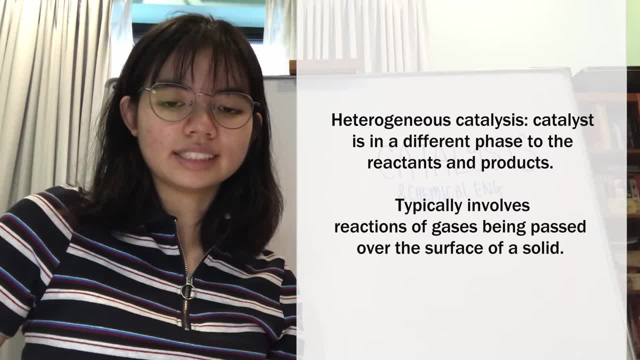 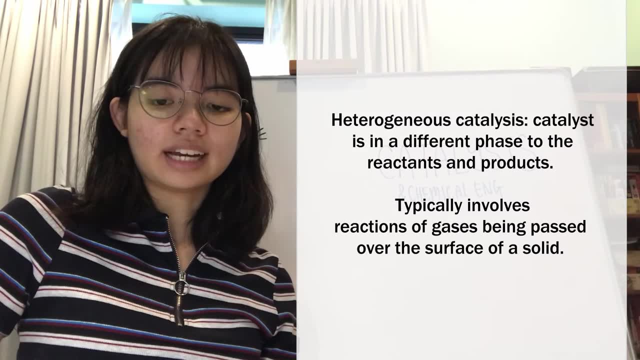 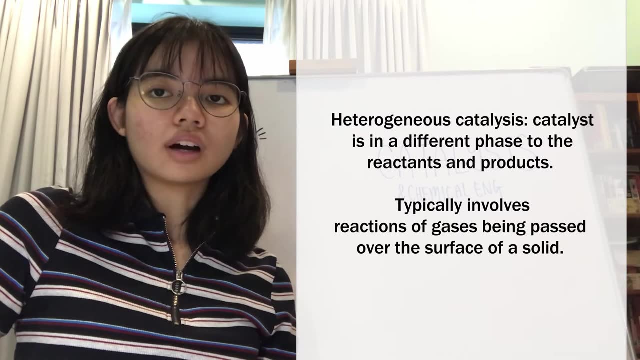 In heterogeneous catalysis, the catalyst is in a different phase or state of matter to the reactants and products. Heterogeneous catalysis is often favored in industry as the catalyst can be easily separated and recovered from the products, although the process is often less specific and allows. 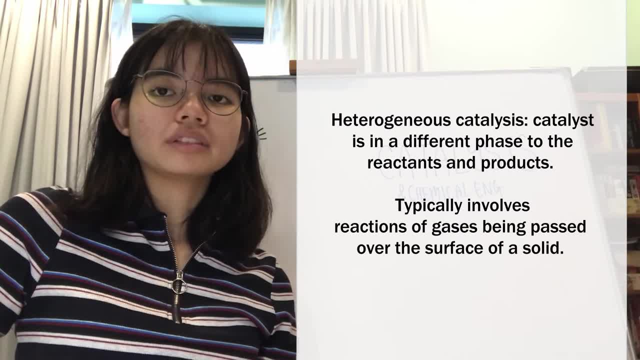 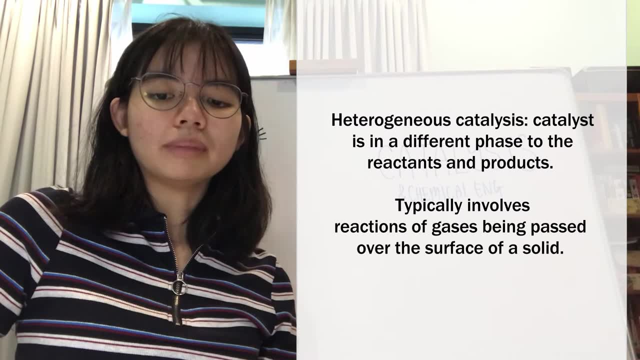 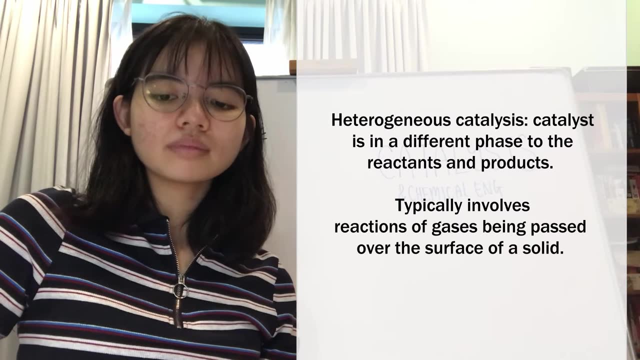 side reactions to occur. The most common examples of heterogeneous catalysis in industry involve the reactions of gases being passed over the surface of a solid catalyst, often a metal, metal oxide or zeolite. A zeolite is a microporous aluminosilicate mineral. 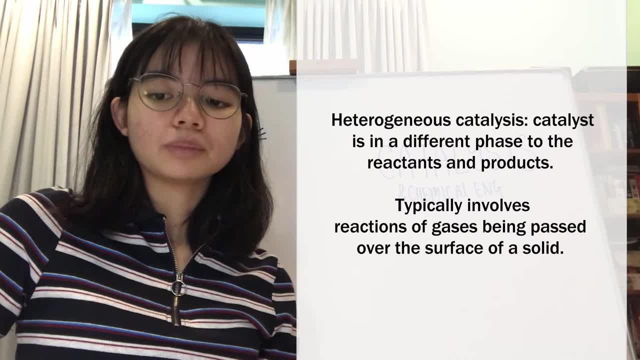 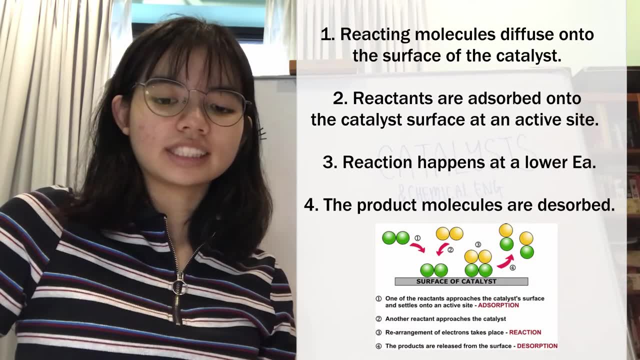 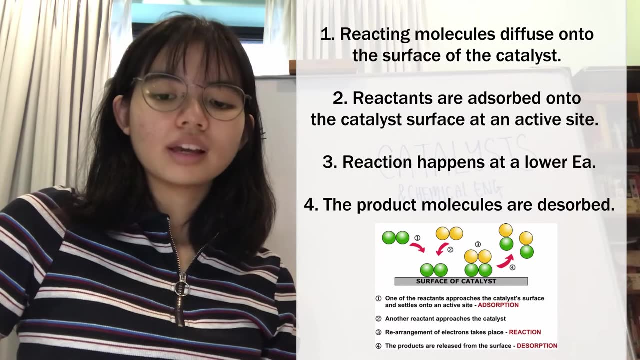 Chemical engineers have to design and oversee structures and machinery, such as purifiers and chemical reactors that enable catalysis to occur on a large scale. So here's how heterogeneous catalysis works, assuming that the reactants are gases and the catalyst is a solid, which is how it normally works in industry. 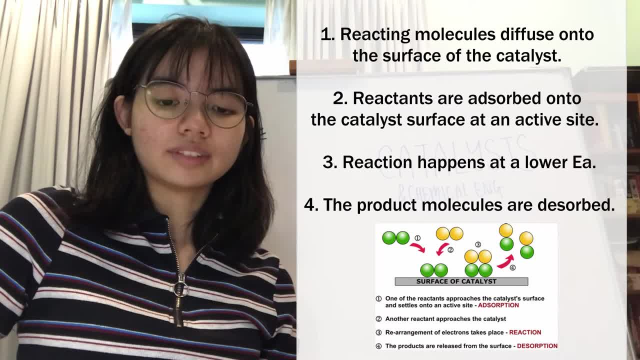 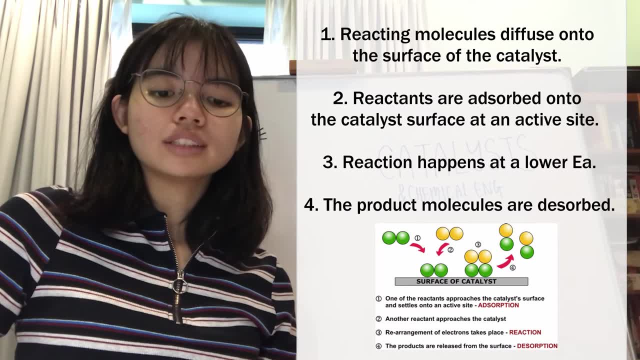 Firstly, the reacting gas molecules diffuse onto the surface of the catalyst. Secondly, the reactants are adsorbed onto the surface of the catalyst at an active site. Adsorption is the adhesion of atoms, ions or molecules from a gas, liquid or dissolved. 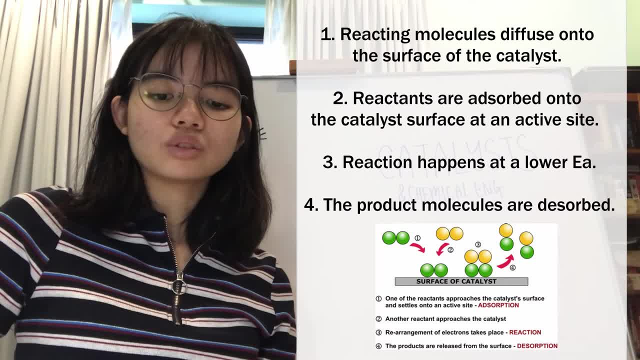 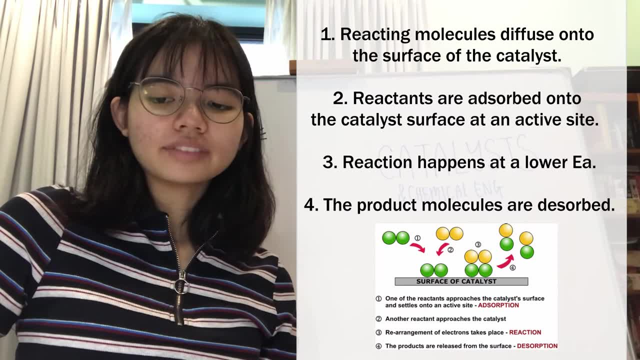 solid onto a surface, creating a film of the adsorbate onto the surface of the adsorbate. Adsorption is separate from absorption. An active site of the catalyst is a place on the catalyst that is adsorbent. So it's not all about absorption. 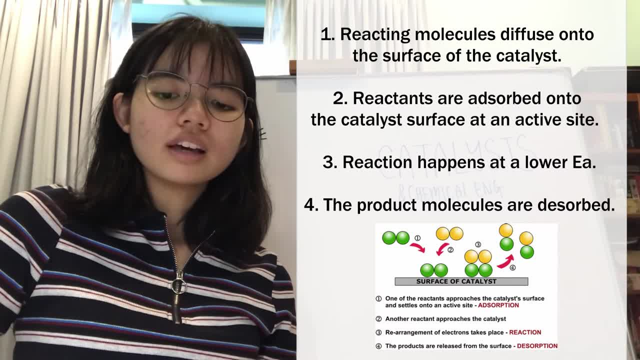 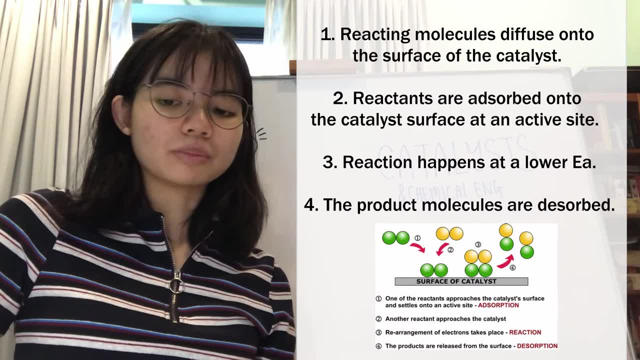 It's also about absorption. especially conducive to adsorption, Physisorption- the formation of weak intermolecular bonds with the atoms of the catalyst, may happen, followed by chemisorption, which is the formation of chemical bonds between the reactant and catalyst. 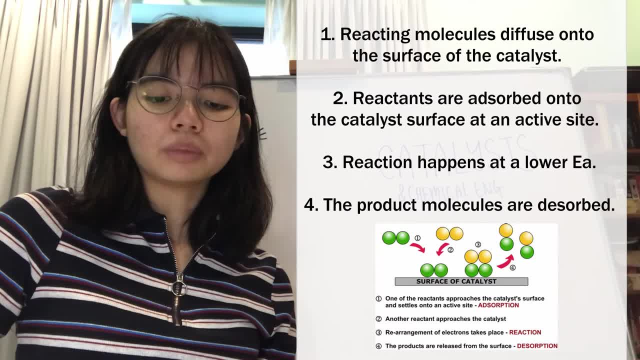 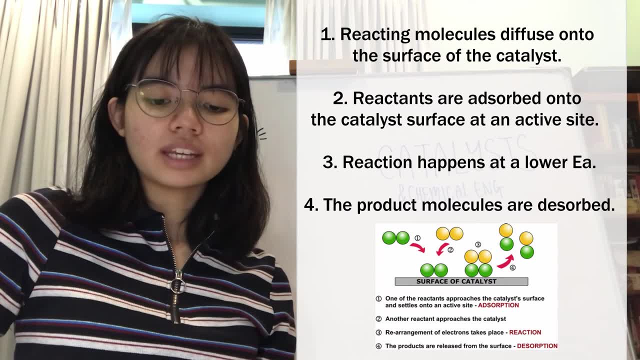 Thirdly, there's an interaction between the surface of the catalyst and reactant molecules, making them more reactive, which might involve an actual reaction with the surface, such as chemisorption or some weakening of the bonds in the attached molecules. The reaction will happen. 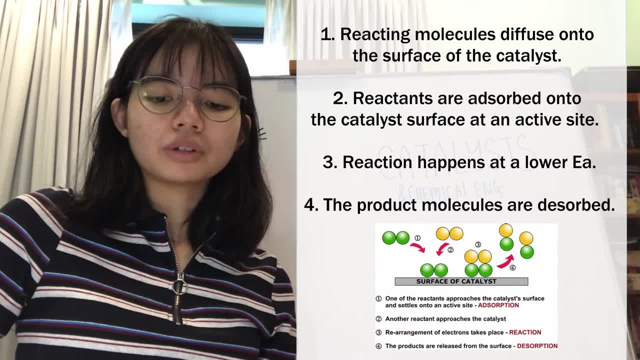 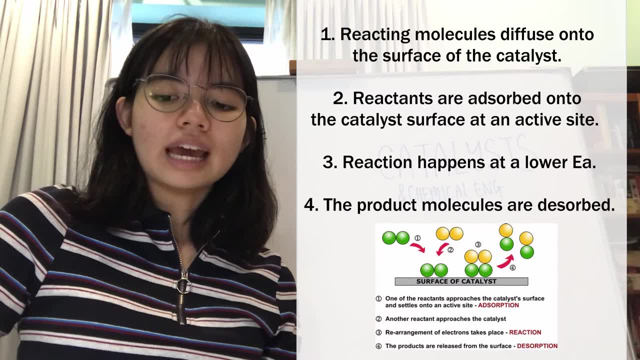 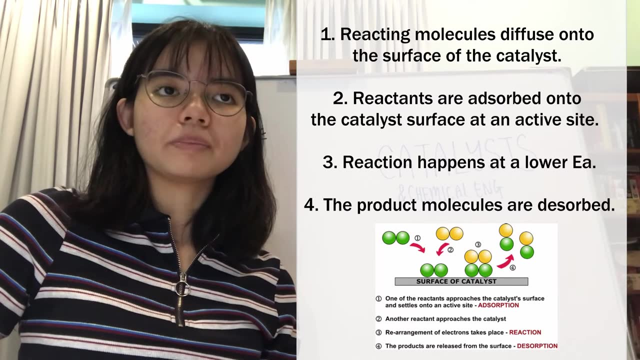 at a lower activation energy pathway, where chemical bonds are broken and formed to bring about the formation of product molecules. Lastly, the product molecules are desorbed and break away from the active site, leaving it available for a new set of molecules to attach to and react on the catalyst, repeating a cycle. 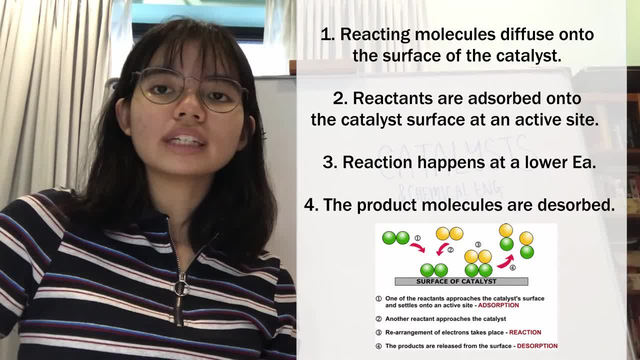 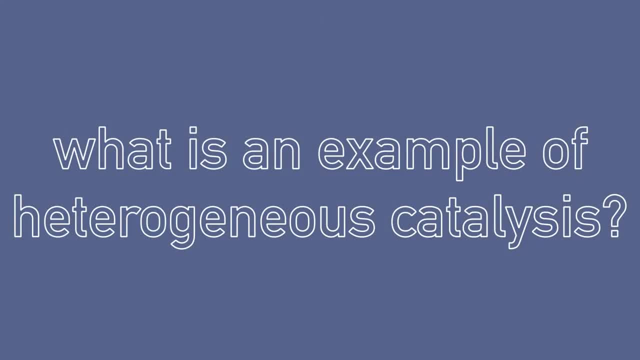 A good catalyst needs to adsorb the reactant molecules strongly enough for them to react, but not so strongly that the product molecules stick more or less permanently to the surface. An example of heterogeneous catalysis in industry is the contact process to produce sulfuric acid. 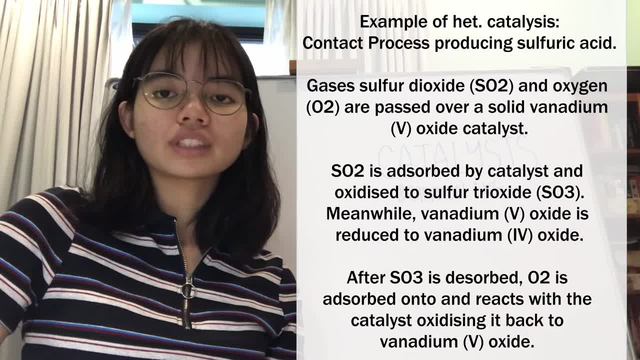 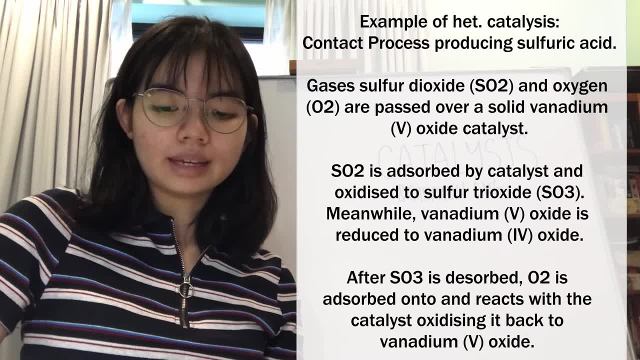 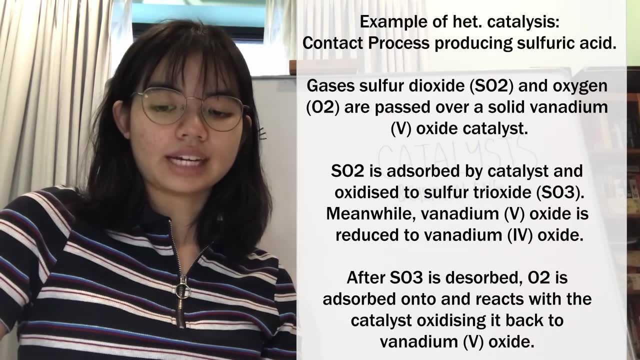 During the contact process. sulfur dioxide has to be first converted into sulfur trioxide. This is done by passing the sulfur dioxide and oxygen onto a solid vanadium oxide catalyst. The sulfide dioxide and oxygen react with the surface of the catalyst in the following series of reactions: 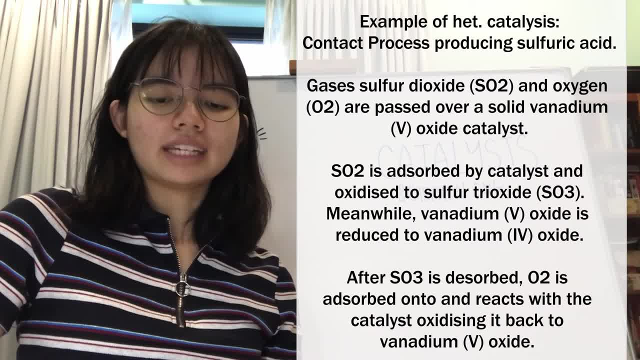 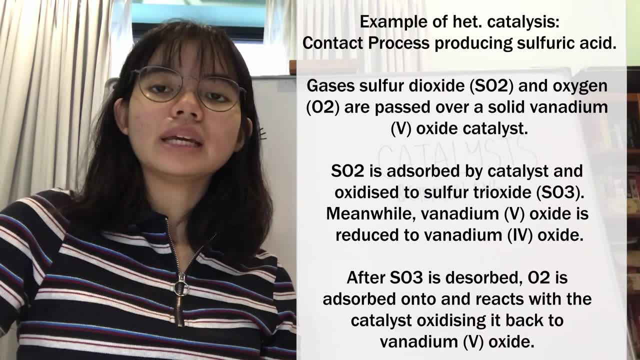 So, firstly, the sulfur dioxide is absorbed by the catalyst, Then it is oxidized to sulfur dioxide trioxide by the vanadium oxide. In the process, the vanadium oxide is reduced to vanadium oxide and the transition state nature of the 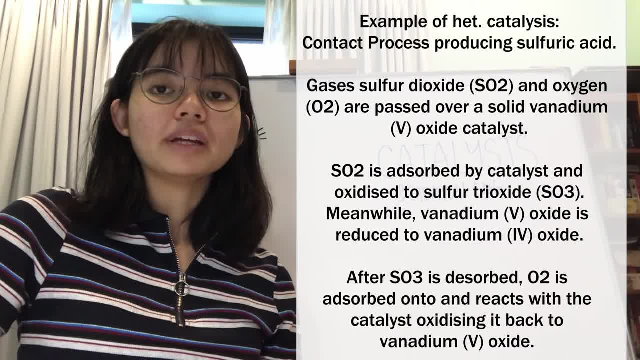 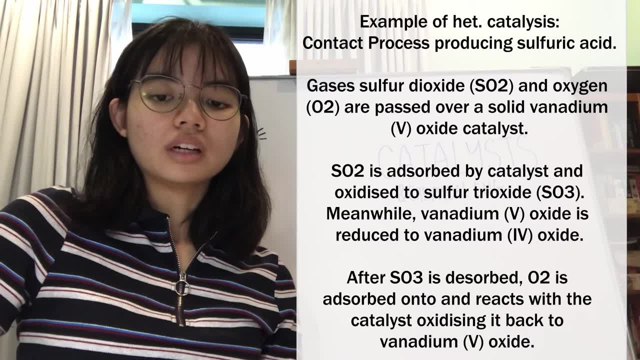 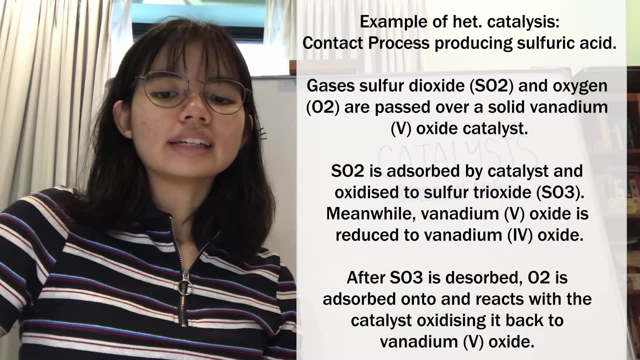 vanadium metal means it can take on multiple oxidation states beneficial for catalysis. After sulfur trioxide is desorbed, oxygen from the air is absorbed onto and reacts with the catalyst, oxidizing it back into vanadium oxide. At the end, the catalyst is chemically the same as it started. 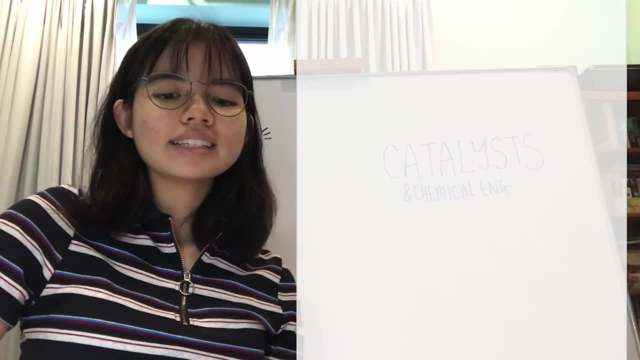 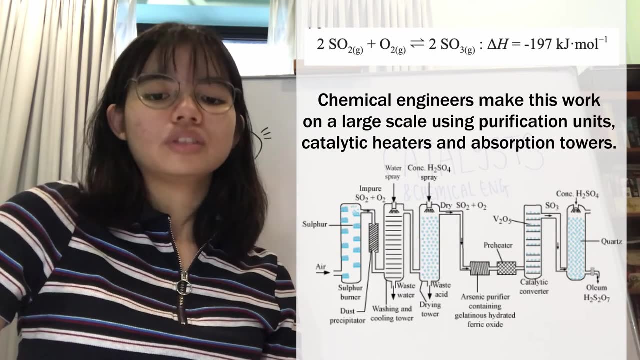 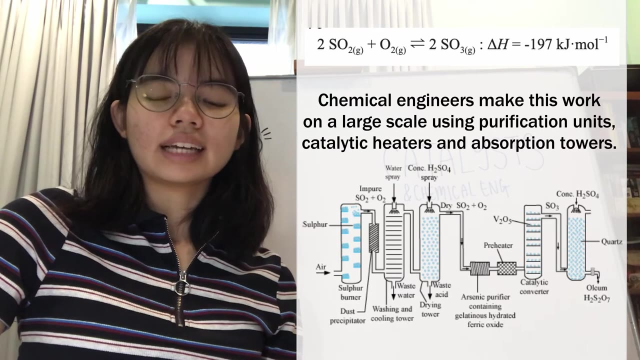 enabling a cycle of catalysis to occur. This seems easy to carry out on a small scale, but chemical engineers work to make it happen on a large scale, using purification units including dusting towers, cooling pipes, scrubbers, drying towers, arsenic purifiers and testing boxes, as well as catalytic heaters, which 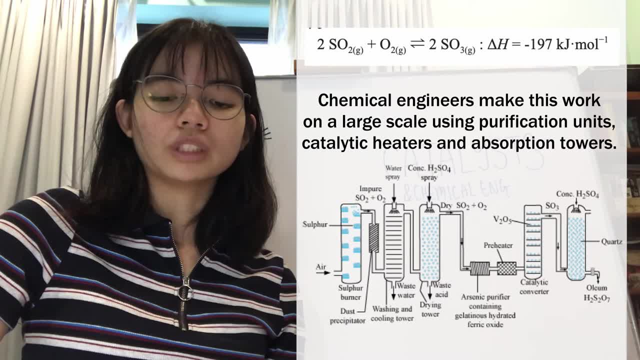 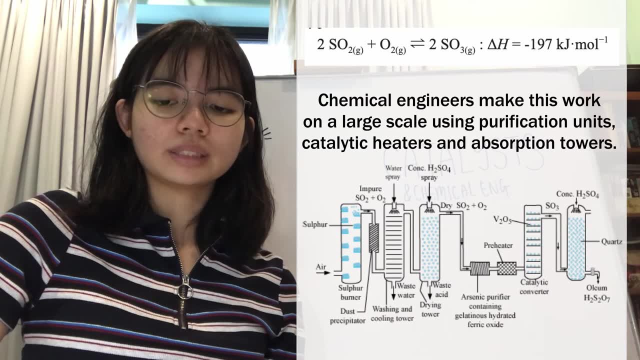 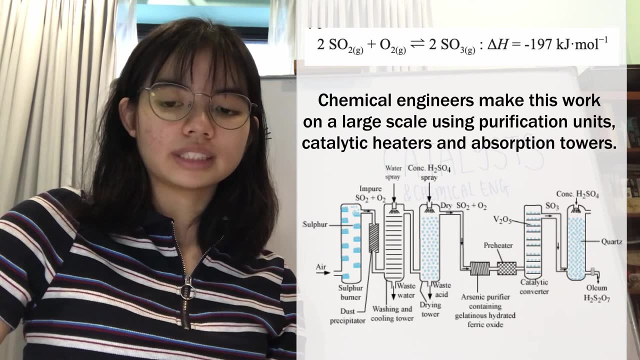 are flameless heaters relying on the catalyzed chemical reaction to produce heat. and finally adsorption towers, which are long vertical columns used in industry for absorbing gases. So the sulfur dioxide needs to be purified in a purification unit to avoid catalyst poisoning or the partial or total deactivation of a catalyst by a. chemical compound that adsorbs onto the catalyst, preventing the reactants from adsorbing Afterwards. the sulfur dioxide is converted into sulfur trioxide in the catalyzed reaction above, which needs to be heated to 450 degrees Celsius using a catalytic heater. Hot sulfur trioxide passes through the heat exchanger and 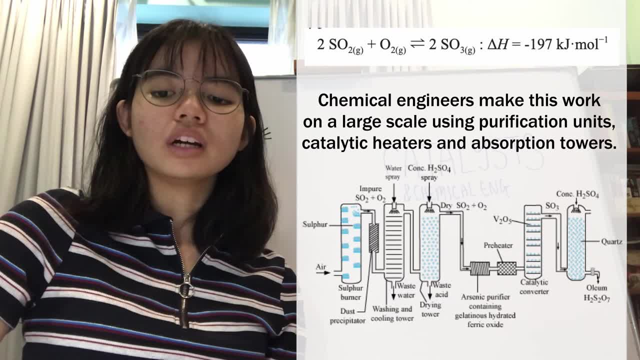 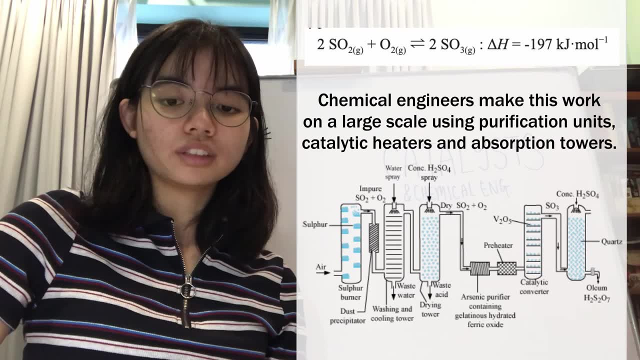 is dissolved in concentrated sulfuric acid in the adsorption tower to form oleum, or H2O7S2,, and this oleum is reacted with water to form concentrated sulfuric acid. Process engineers, which are types of chemical engineers, implement process. 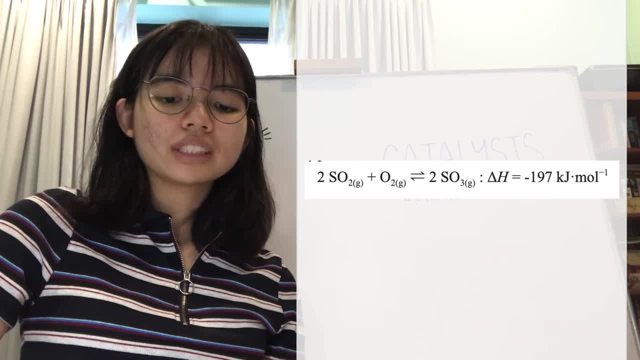 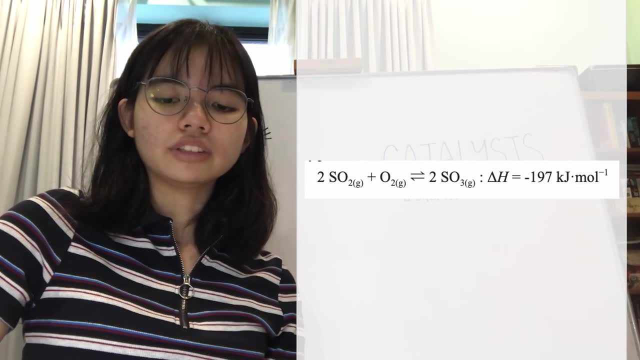 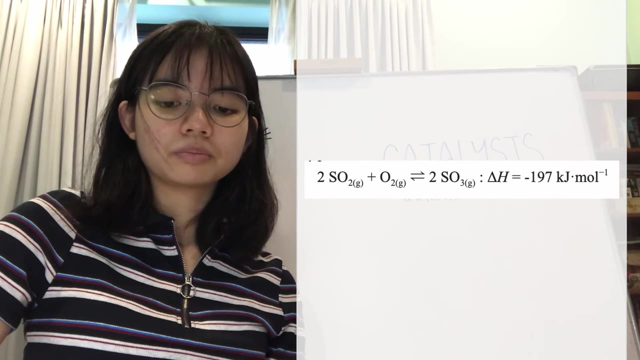 improvements to reduce cost and increase efficiency. They are the ones devising and overseeing the above process. They work to reduce operational costs, for example striking a balance between yield and reaction rate. If we look at the reaction between sulfur dioxide and oxygen according to Le Chatelier's. principle, a lower temperature should be used to shift the chemical equilibrium towards the right, increasing the percentage yield. However, too low of a temperature will lower the formation rate to an uneconomical level. So to increase the reaction rate, process engineers decided that high temperatures. 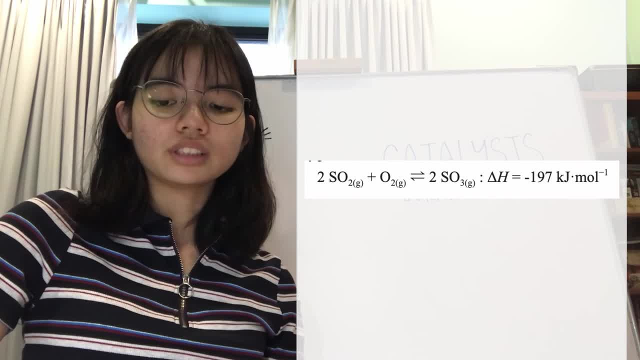 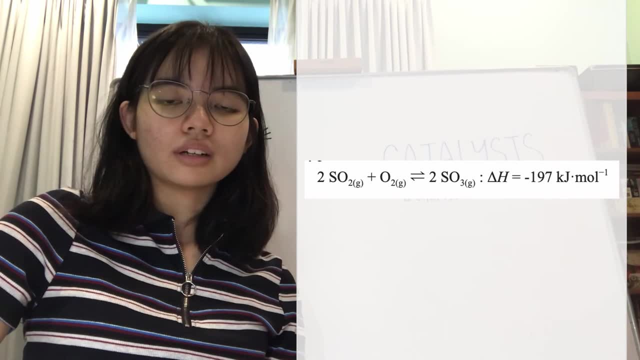 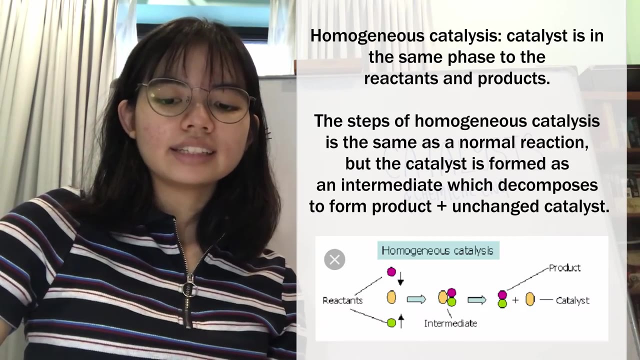 of 450 degrees Celsius, medium pressures of one to two atmospheres and a vanadium oxide catalyst will be used to increase the reaction rate. The reaction rate will be reduced to a to ensure an optimal or more than 95% conversion In homogeneous catalysis. the catalyst is in the same phase or state of matter to the 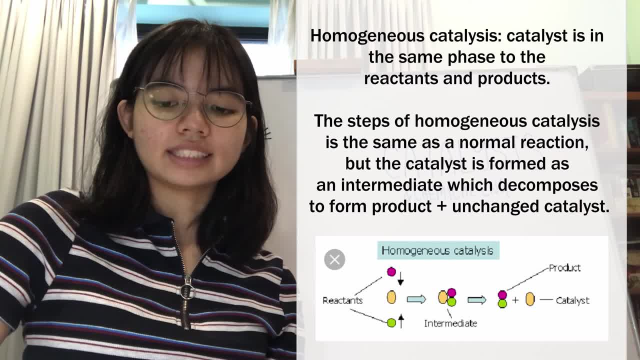 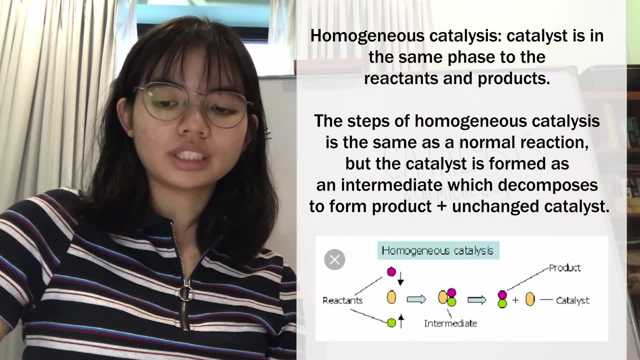 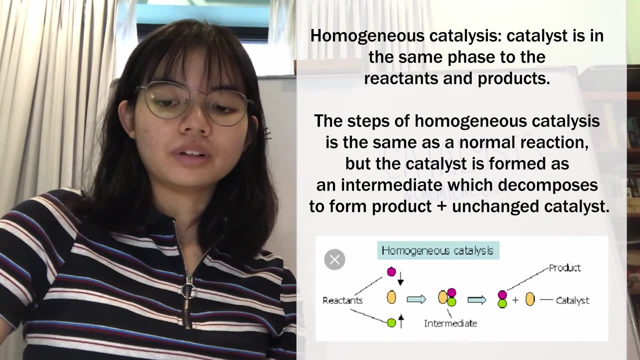 reactants and products. An advantage of homogeneous catalysis is that the catalyst mixes into the reaction mixture, allowing a very high degree of interaction between the catalyst and reactant molecules. However, unlike heterogeneous catalysts, the homogeneous catalyst is often irrecoverable. 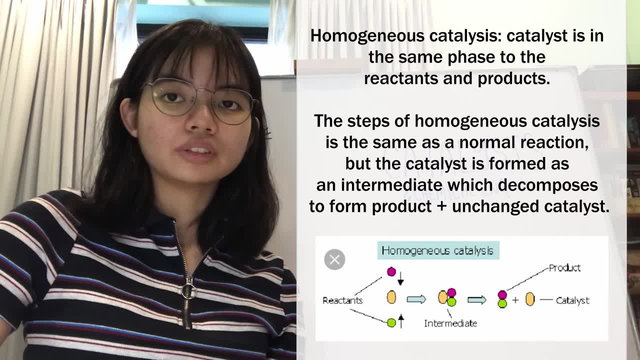 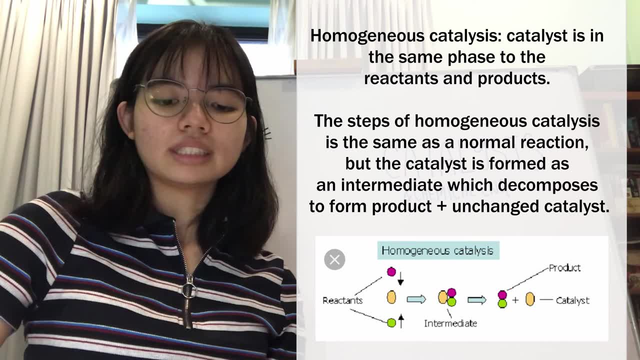 after the reaction has run to completion, so they are less often used in industrial settings. The steps of homogeneous catalysis is just the same as a normal reaction, but the catalyst is formed as an intermediate during the reaction, which then decomposes to form the product. 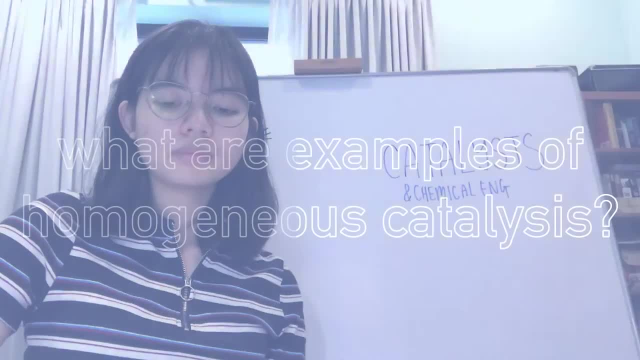 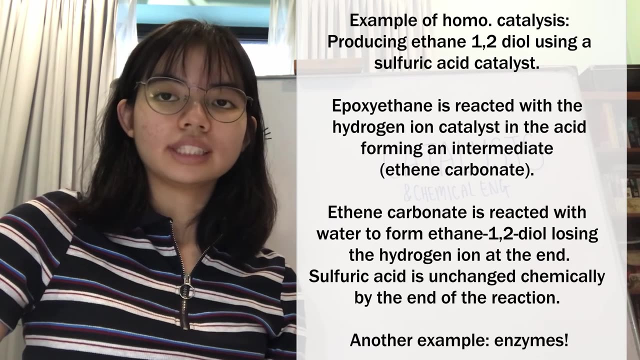 and the unchanged catalyst. as we can see in the diagram, An example of homogeneous catalysis is the manufacture of ethane-1,2-diol using a sulfuric acid catalyst. Ethane-1,2-diol is used as an antifreeze injector. 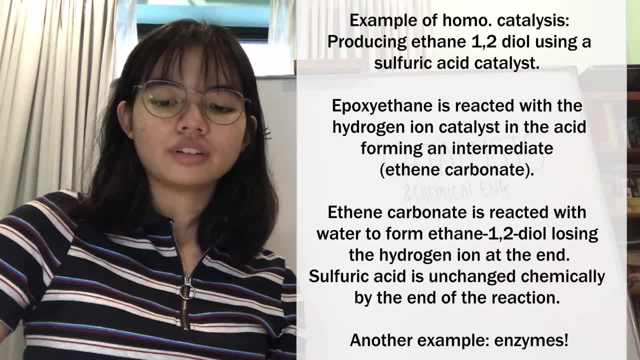 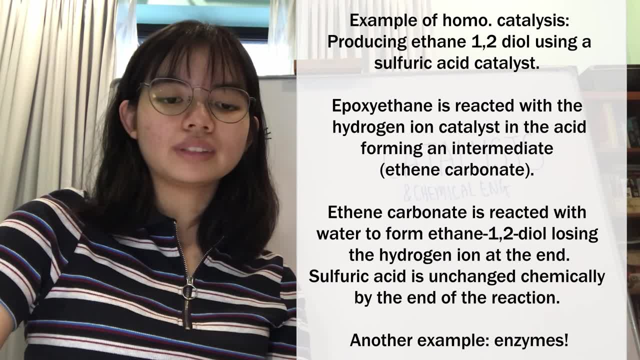 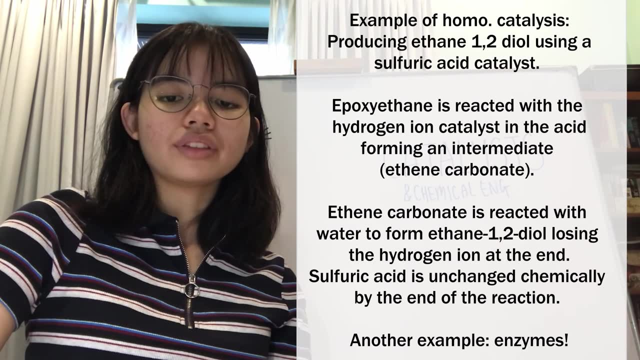 It is added to cooling water to prevent it from freezing under very cold conditions. In the homogeneous catalysis epoxy, ethane is reacted with the hydrogen ion catalyst and the sulfuric acid to form an intermediate step, producing 1,3-dioxylan-2-one or ethene. 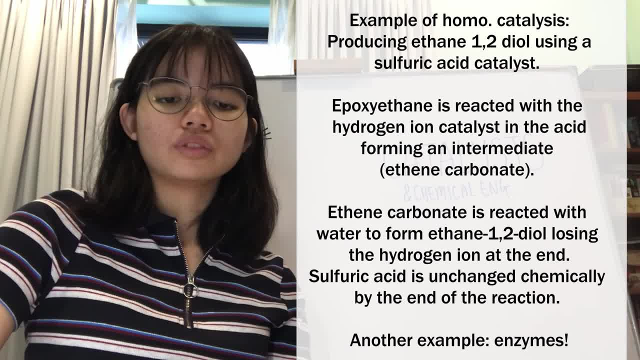 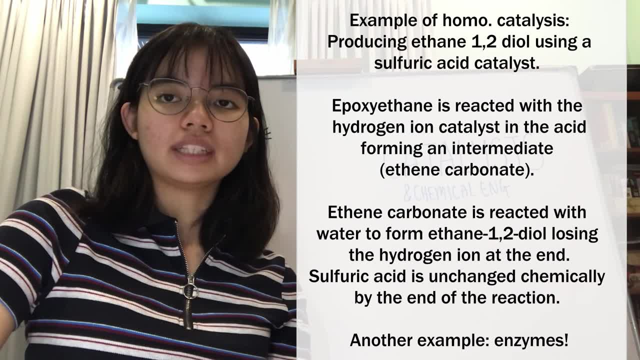 carbonate. Ethene carbonate is then reacted with water to form ethane-1,2-diol, losing the hydrogen ion at the end, showing that the sulfuric acid remains unchanged chemically by the end of the reaction. After leaving the reactor, the product is distilled at lower pressures to remove water. 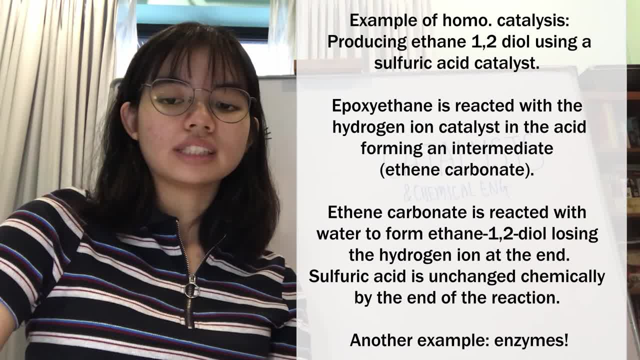 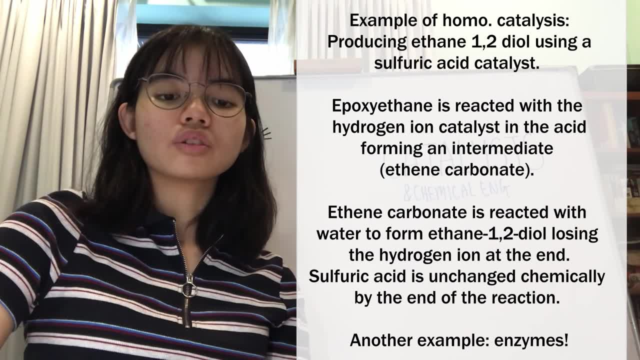 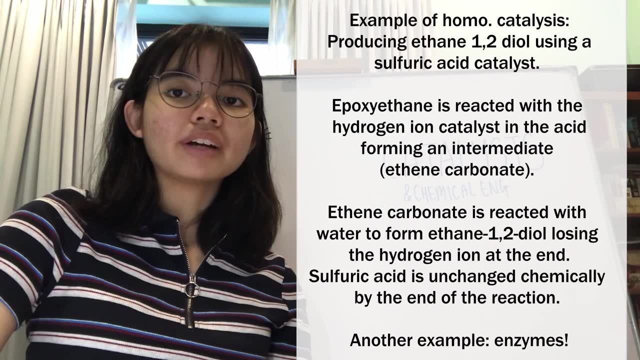 which is returned to the reactor, and the ethane-1,2-diol is then purified through vacuum distillation. Heat from the reactor is used to heat the distillation columns, and this process is also overseen by process engineers. Another example of homogeneous catalysis is biocatalysis with enzymes, which I mentioned. 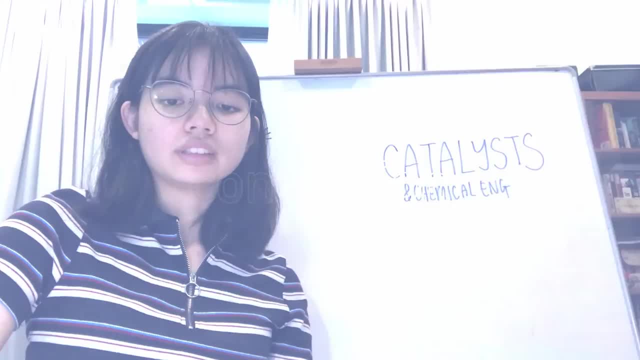 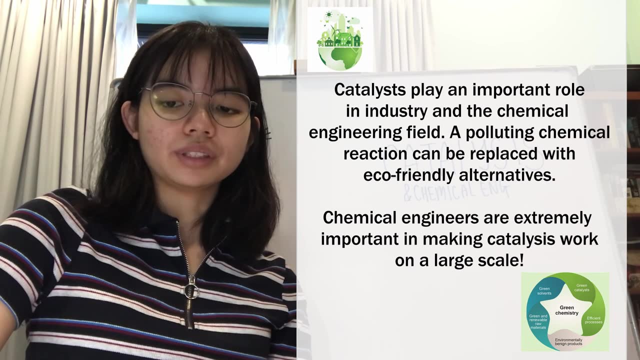 in the biotechnology video two weeks ago. Overall catalyst-free. catalysts can be found in the bioprocessing process or in the bioprocessing process. They play an important role in industrial research, the chemical industry and the chemical engineering field. 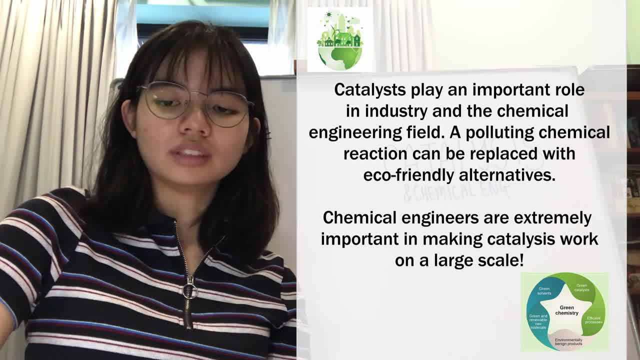 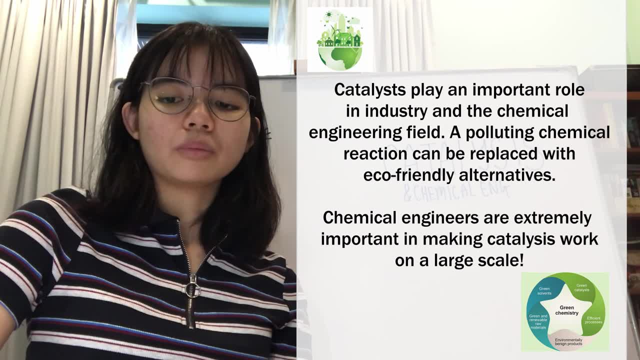 Different catalysts are in constant development to fulfill economic, political and environmental demands. When using a catalyst, it is possible to replace a polluting and high-cost chemical reaction with a low-cost and more environmentally friendly alternative. Today and in the future, this is vital for the chemical industry. 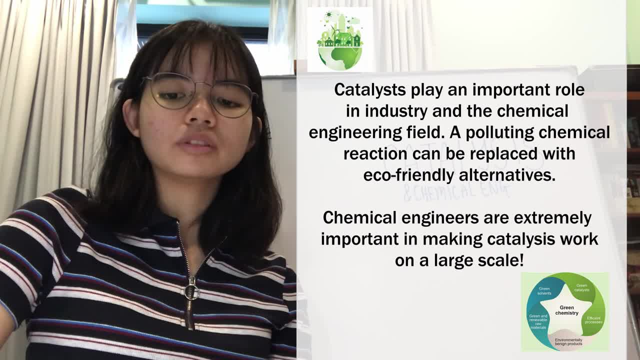 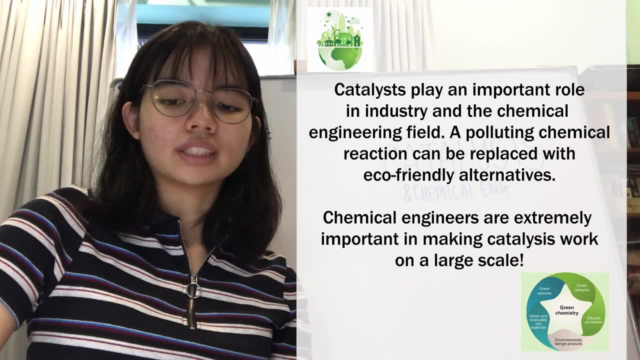 And chemical engineers, by using knowledge of how heterogeneous and homogeneous catalysis works, are instrumental in making the chemical industry a better place to work. Thank you. Industrial catalysts work on a large scale by overseeing and designing processes and structures for catalysis to happen efficiently. 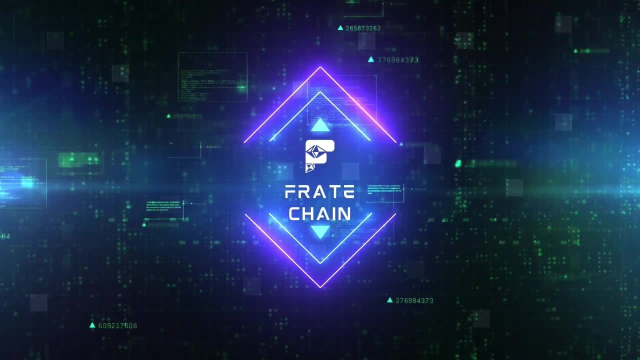 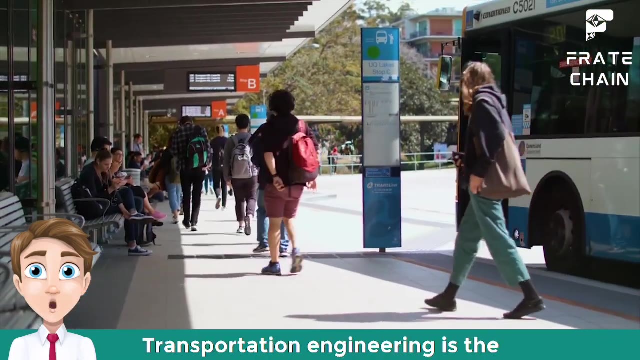 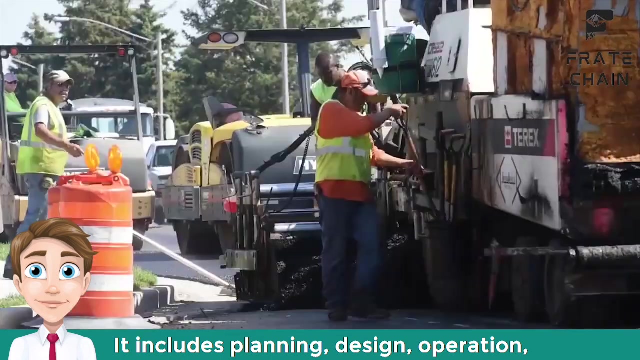 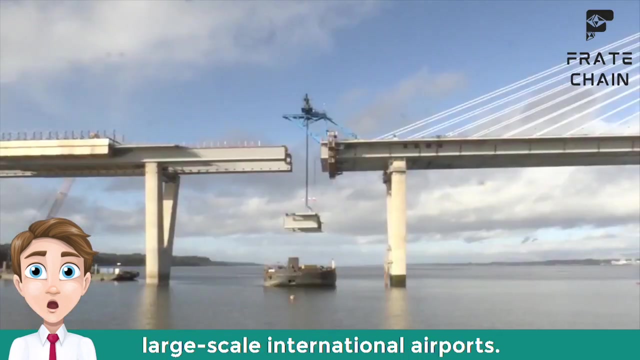 What is transportation engineering and what do they do? Transportation engineering is the application of technology and scientific principles to transportation systems. It includes planning, design, operation and maintenance. Transportation engineers work on a variety of projects, from small-scale local roads to large-scale international airports. 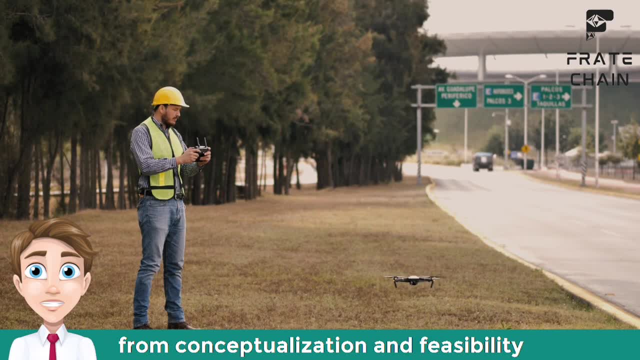 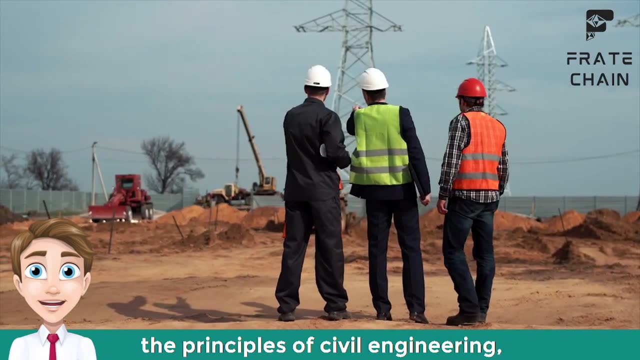 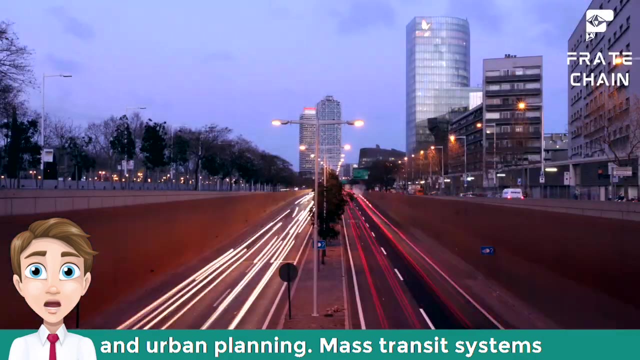 They are involved in every project stage, from conceptualization and feasibility studies to construction and operations. Transportation engineering is a multidisciplinary field that draws on the principles of civil engineering, mechanical engineering, electrical engineering, industrial engineering and urban planning, Mass transit systems, highway systems, airports. 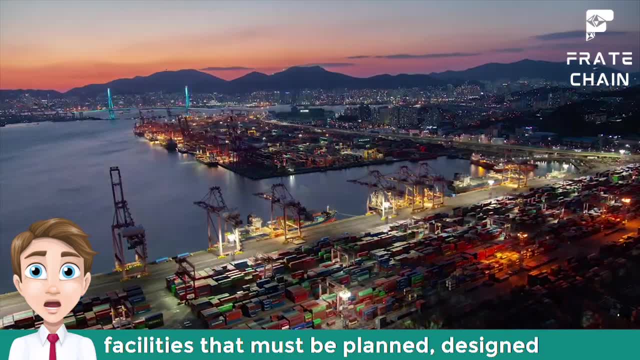 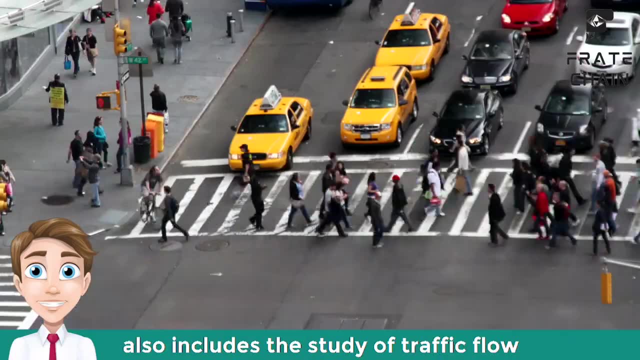 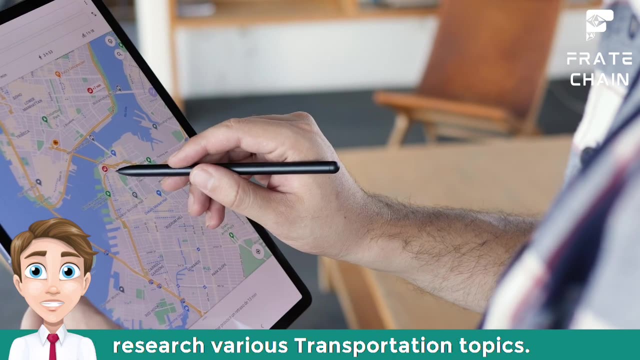 and maritime ports are all examples of transportation facilities that must be planned, designed and maintained by transportation engineers. Transportation engineering also includes the study of traffic flow and management, as well as roadway safety. Transportation engineering faculty members at many universities also research various transportation topics. If you want to learn more about the other types of transportation,